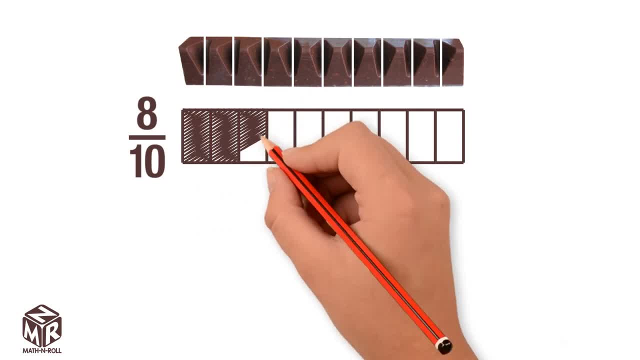 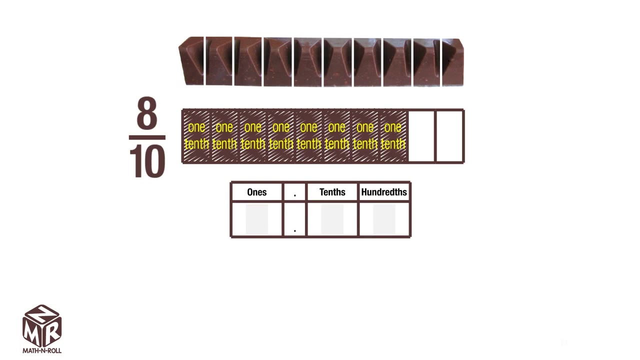 Let's shade 8 tenths of the model. Each part represents 1 tenth. Use a place value chart to show 8 tenths. We put a zero in the ones column because we don't have a full part. We put an eight in the tenths column because we have eight shaded tenths. 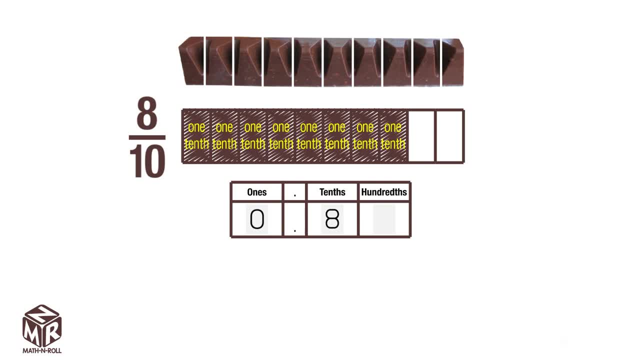 So the fraction 8 over 10, or 8 tenths can be written as a decimal, as 8 tenths. We can also use a number line Label the number line with decimals that are equivalent to the fractions 0 tenths, 1 tenth, 2 tenths. 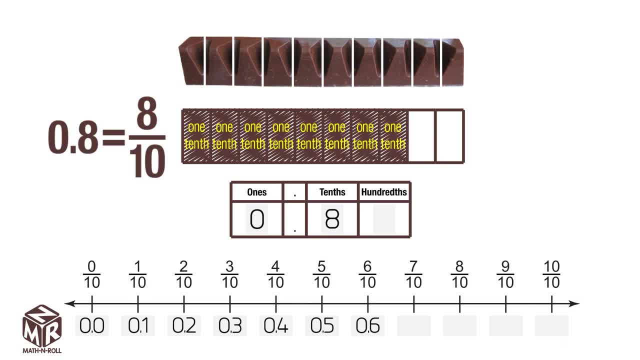 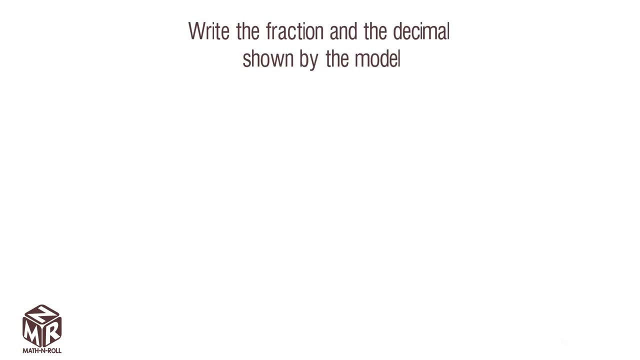 and so on. Locate the point 8 over 10.. The fraction 8 over 10, or 8 tenths is equivalent to the decimal 8 tenths. Write the fraction and the decimal shown by the model. We have a model consisting of 10 parts. 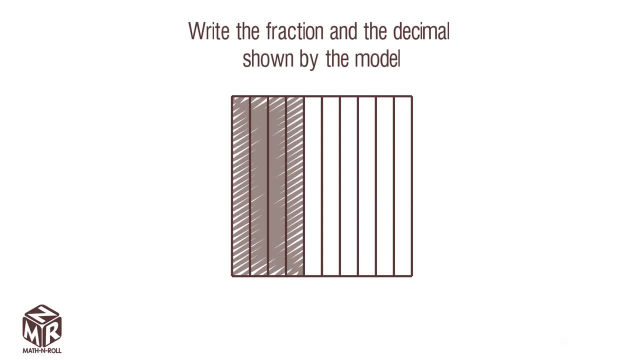 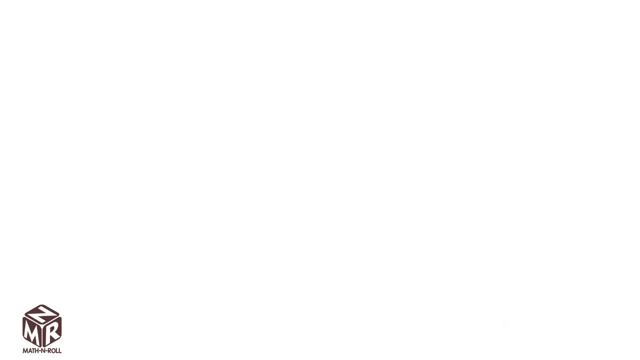 Each part represents 1 tenth. 4 out of 10 tenths are shaded, so we write the fraction as 4 over 10, or 4 tenths. The decimal is also 4 tenths. Let's try another example. 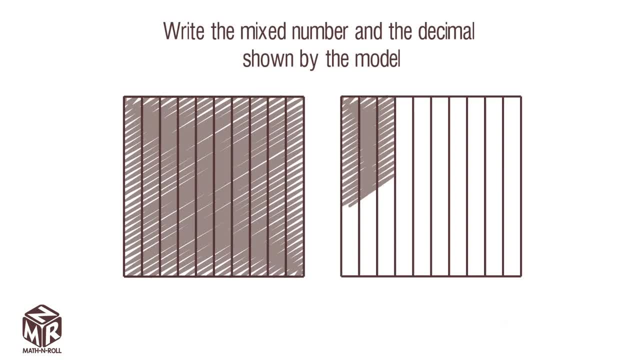 Write the mixed number and the decimal shown by the model. This time we have 1 whole and 3 out of 10 parts, So we write the mixed number as 1 and 3 tenths. The decimal is 1 and 3 tenths, or 1.3.. 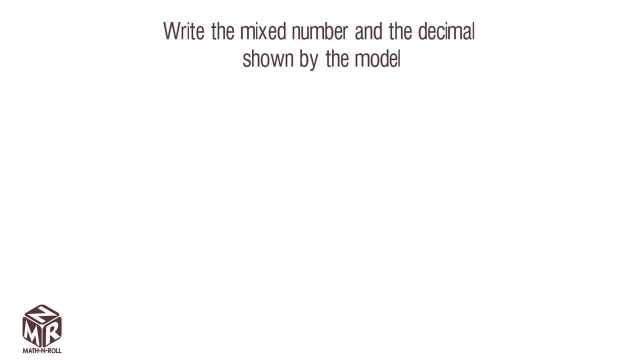 Let's try another example. Write the mixed number and the decimal shown by the model. On the left side of the number line we see 3 and 0 tenths or 3.0.. On the right side of the number line we see 3 and 5 tenths or 3.5. 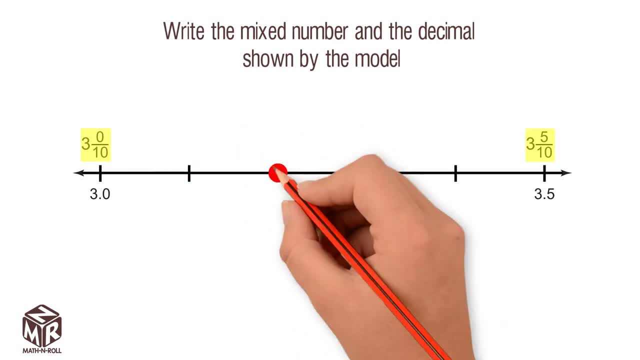 Let's try another example. In between there are 5 parts. Each part represents 1 tenth. So the first point to the right of 3.0 is 3 and 1 tenth. To find the next point, we add 1 tenth.